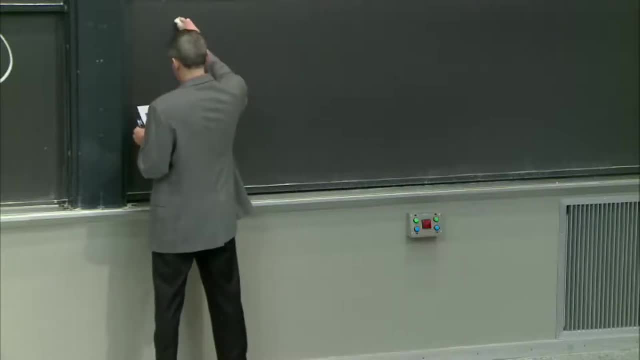 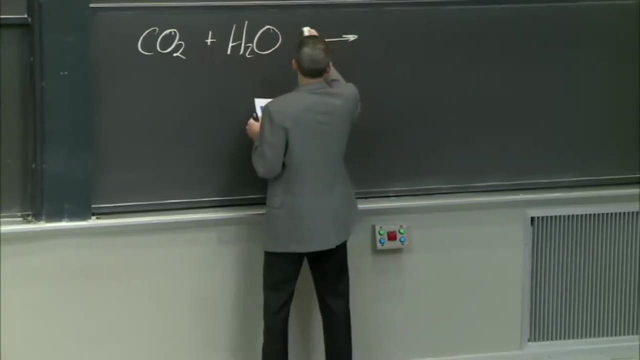 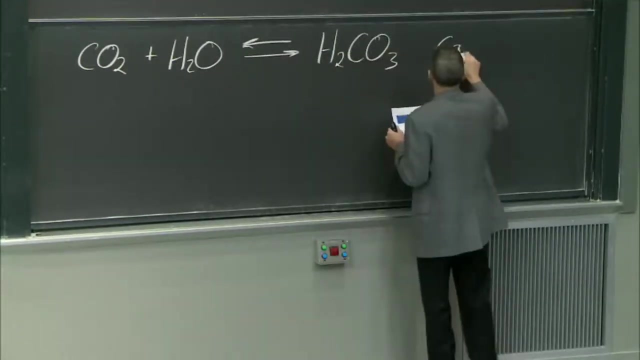 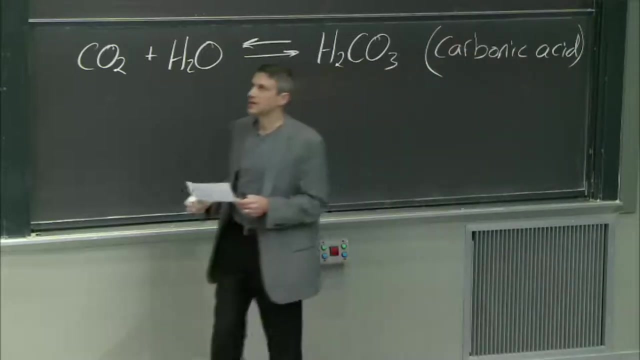 Say that at the Thanksgiving table, You'll be very popular. We said CO2 plus H2O. This goes- Oh, it finds some equilibrium to H2CO3.. Now this is called carbonic acid. This is called carbonic acid. 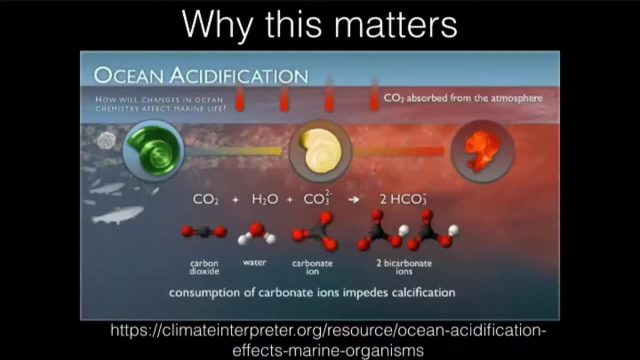 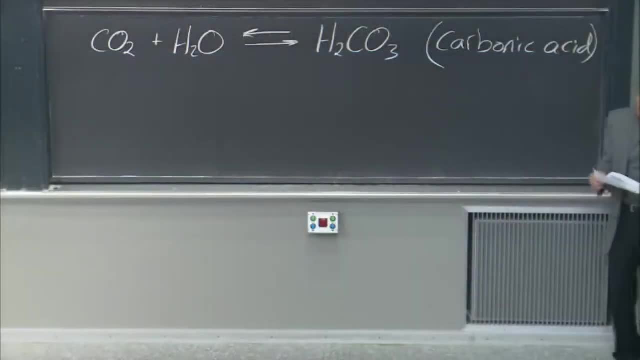 There's the terrapot up there And there's a reaction that's really relevant, that you'll see from the ones we're about to write down why? Because the thing is what happens to carbonic acid. Well, carbonic acid also goes through a dissociation. 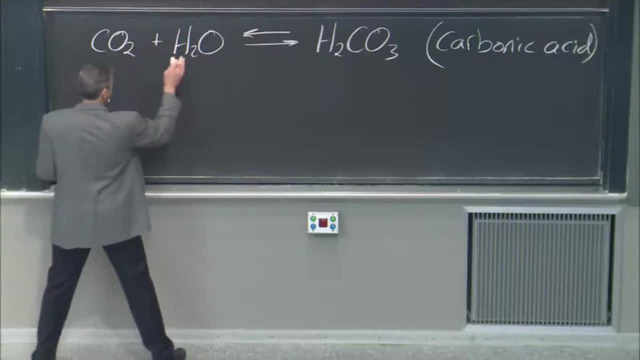 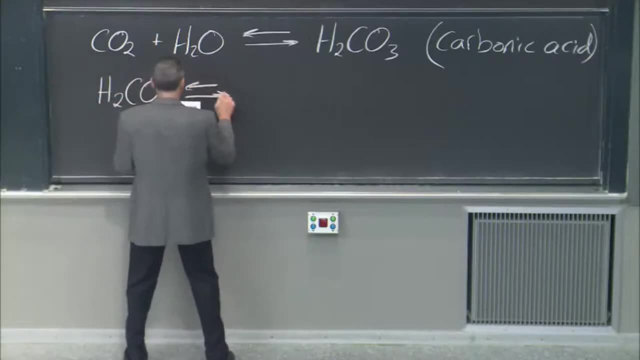 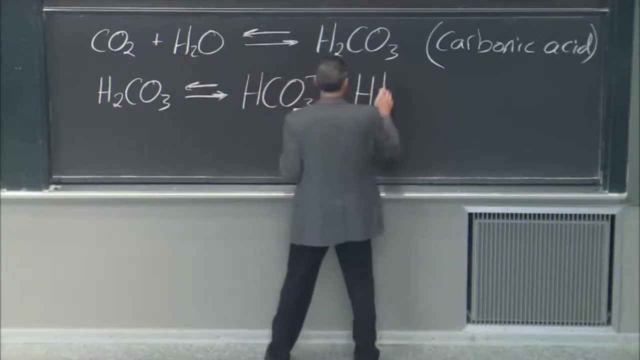 It's a solution reaction, So carbonic acid. so this is CO2 dissolving in water. Now we made carbon, So carbonic acid goes like this: OK, it goes into HCO3 minus plus H plus. Now here's the thing. 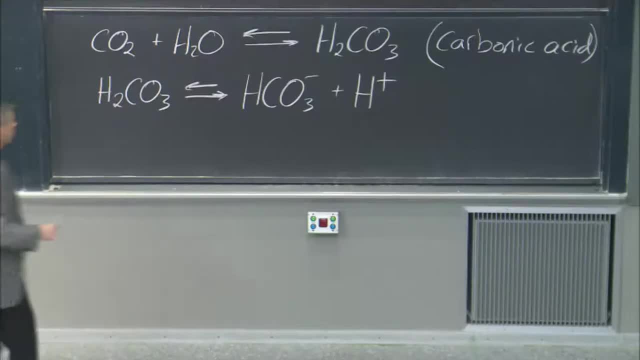 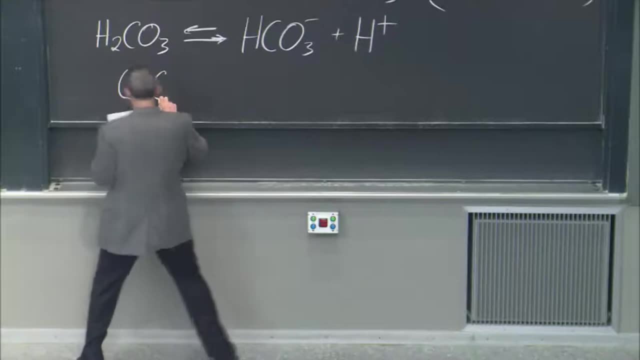 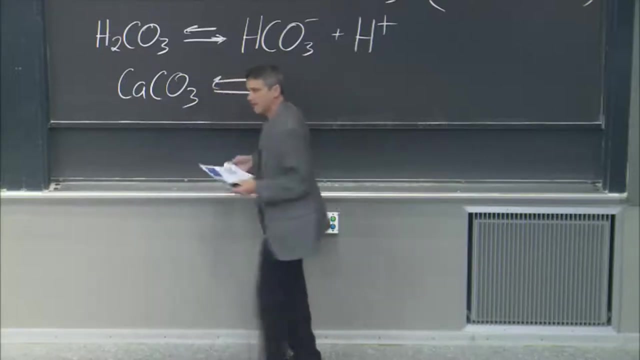 OK, what is the shell made of? Well, the shell that's dissolving in its, you know like, the core material is calcium carbonate, So that's CaCO3.. That's the shell. And the shell also has an equilibrium reaction. 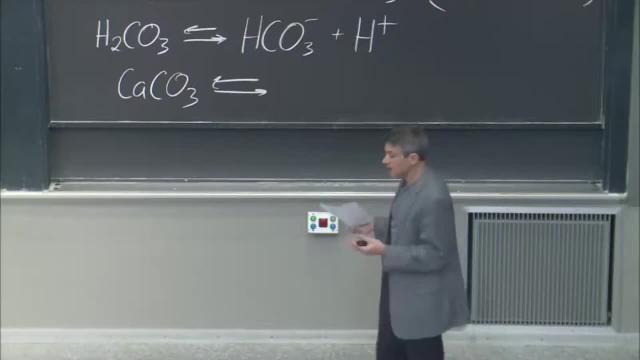 That happens, The shell of a sea creature is in dynamic equilibrium with the ocean, And so it's going like this. It's going to well OK: Ca2 plus and CO3 2 minus, And OK, but the thing is it has an equilibrium constant. 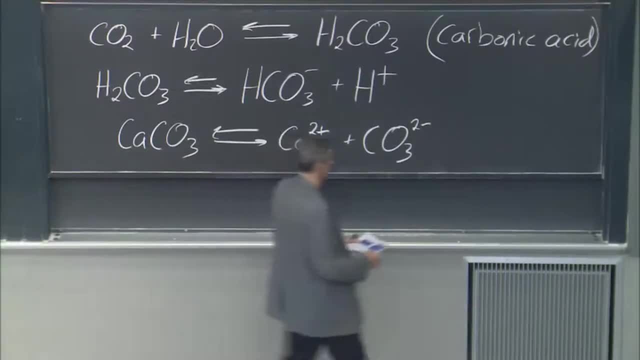 All these have equilibrium constants. So like, for example, for this one, the Ksp, the solubility product constant, because this is a solid, This is a solid shell Solid going to ions in aqueous solution. So the Ksp for that is somewhere around 5 times 10. 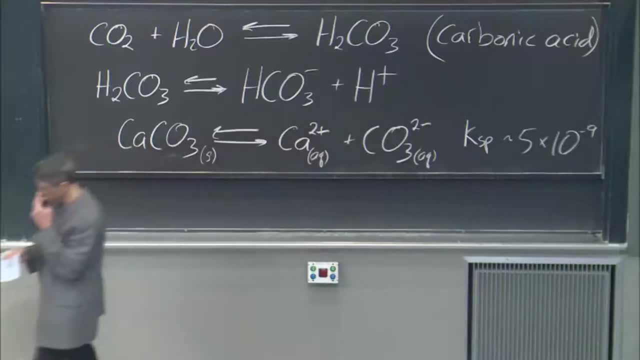 to the minus 9th. 5 times 10 to the minus 9th. Yeah, but here's the thing. We just went through this: If I consume one of these or change the concentration of one of these and not the other, we just did this. 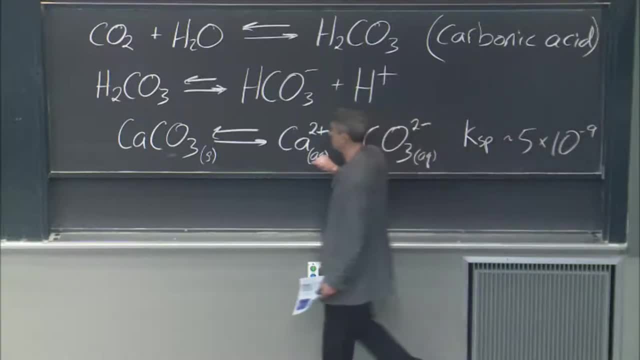 If I change the concentration, if I consume any of these, then I might drive the reaction, Consume or produce. If I change any of these independently, I'm going to drive the reaction because that's how we keep to our K. That's what Le Chatelier's 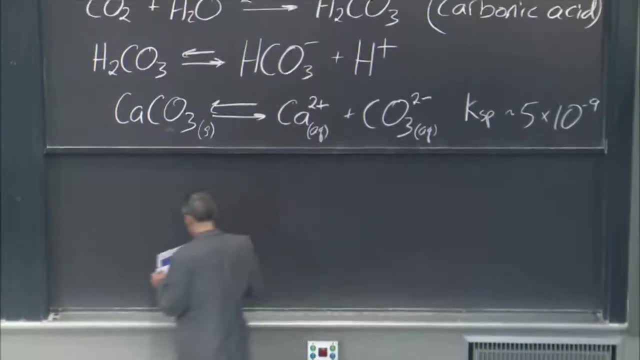 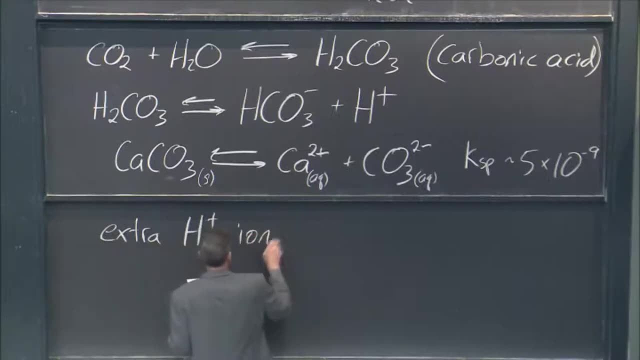 principle tells us. And so what ends up happening is you've got the extra H plus ions, So these are ions in solution. Where did they come from? They came from the CO2, giving us carbonic acid, which then gave us H plus. 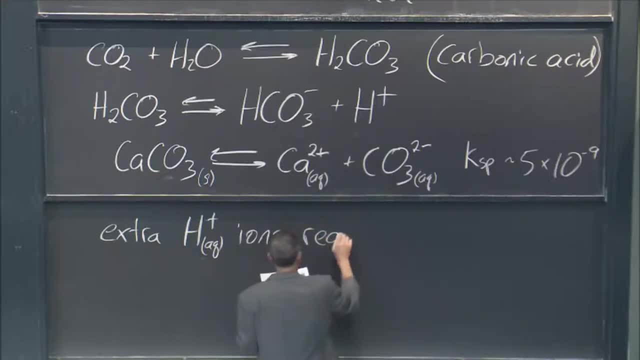 Those are what I'm talking about. Well, they react with the CO3 minus, CO32 minus. So this lowers the CO32 minus concentration near the shell. And if I lower this, because I've taken some of this now and I've reacted it, so now I've got less of it- 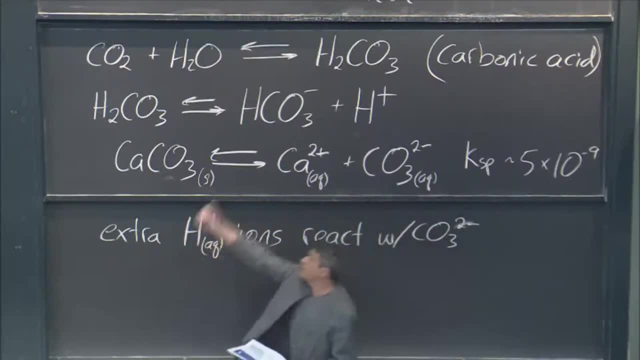 And because of what we just saw, if I've got less of this, you're going to drive this way, which is going to dissolve more of the shell. That's why this works. That's why this happens. Works sounds like a positive thing. 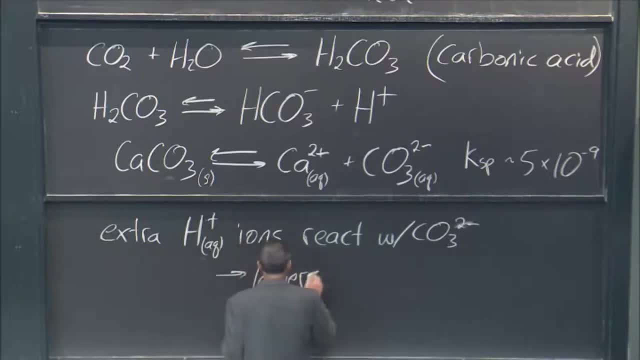 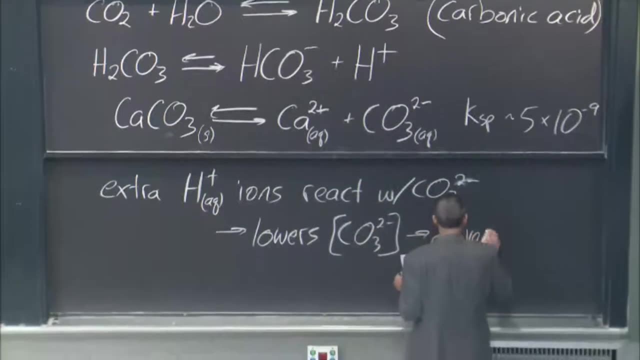 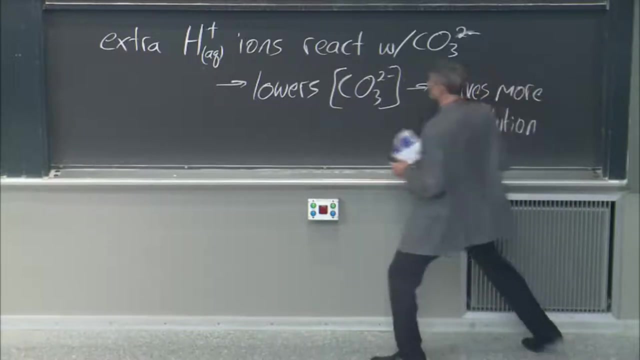 So this lowers the concentration of CO32 minus And that drives more dissolution. That is what's happening, And we now can understand it in terms of the concepts that we've just learned. Historically, I mentioned 50 million years. Actually, by some accounts, it's 300 million. 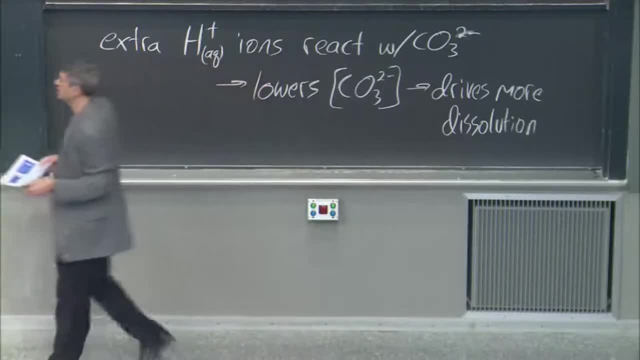 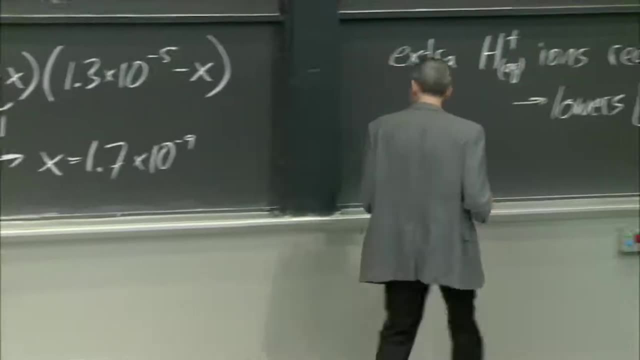 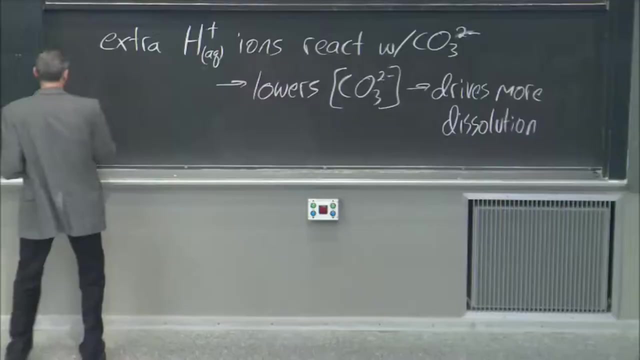 It depends on which studies you read, But for at least 50 and maybe as much as 300 million years, the ocean has had a pH of 8.18.. Now, where's the Oh yeah? So let's just say last oh: 50 to 300 million-ish years. 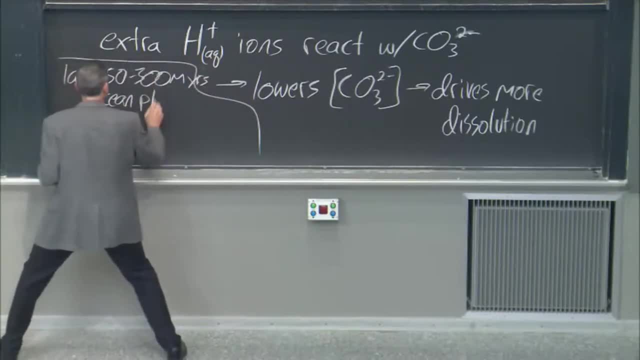 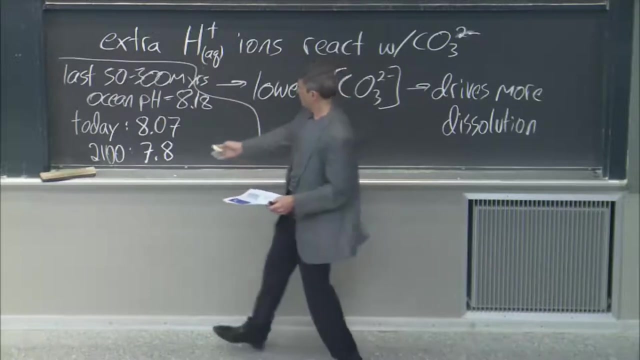 the ocean pH. pH was 8.18. And today it's 8.07.. And the prediction is that in 2100, it will be 7.8.. Now, as we will see in a little bit, what's pH?